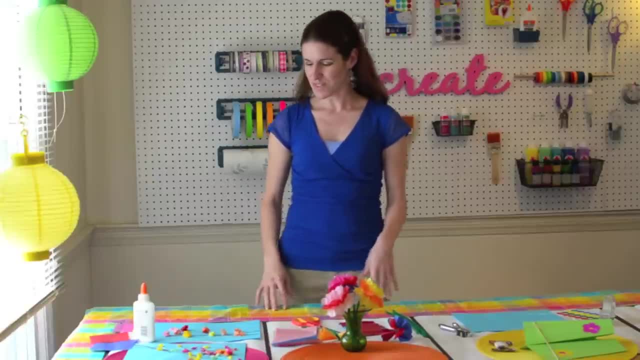 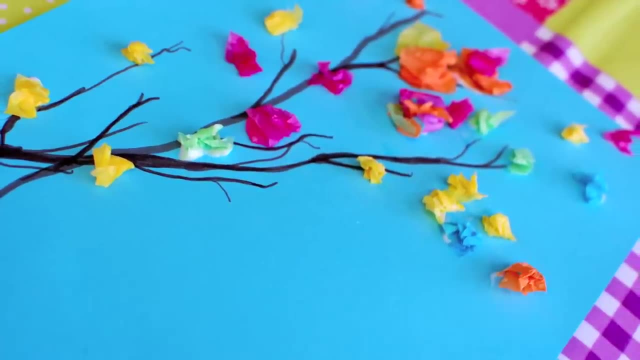 all those and hopefully make some memories for you and your kid. This first project is a branch project that I did with different colored tissue paper and it just looks like a nice colorful branch on a windy spring day. So what you do is start off with a piece of 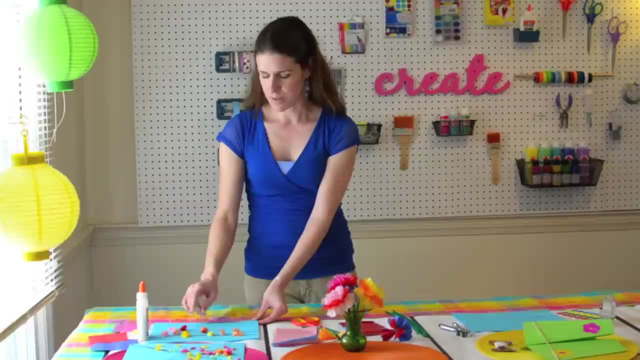 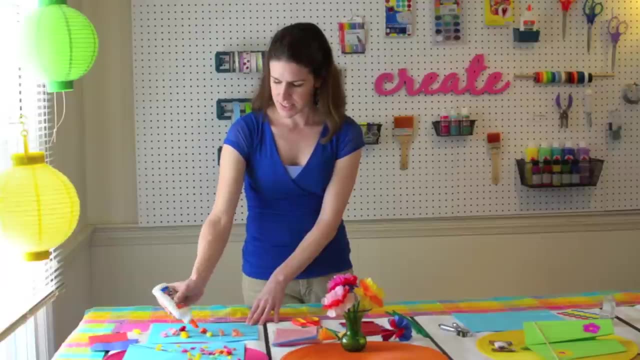 construction paper and just take a marker and go ahead and make a branch on there just for your child to use as a guide, And then invite your child over to glue on little pieces of tissue paper So they can go ahead and rip up the pieces of tissue paper themselves. 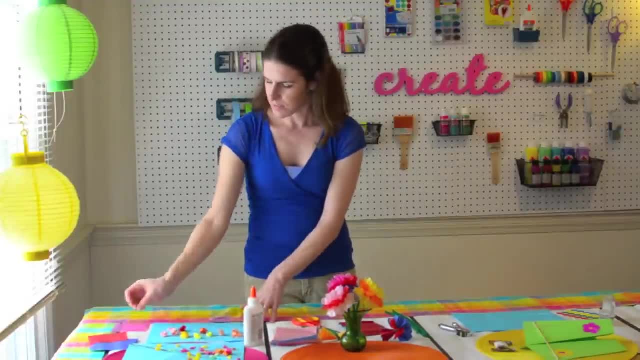 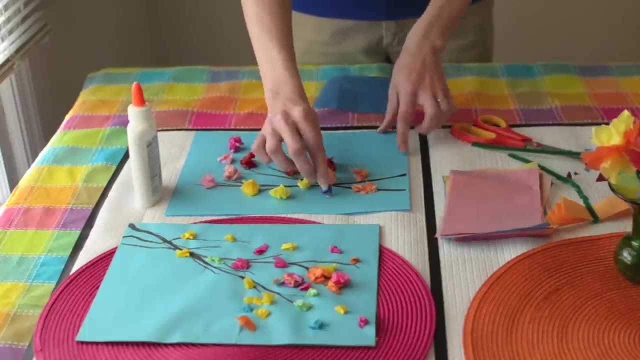 and then just scrunch them up into little blossoms. And what I like about this project is there's really no wrong way to do it. If the blossoms are off of the branch, for instance, it just looks like they're taking off in the wind. So just a nice way for little kids to 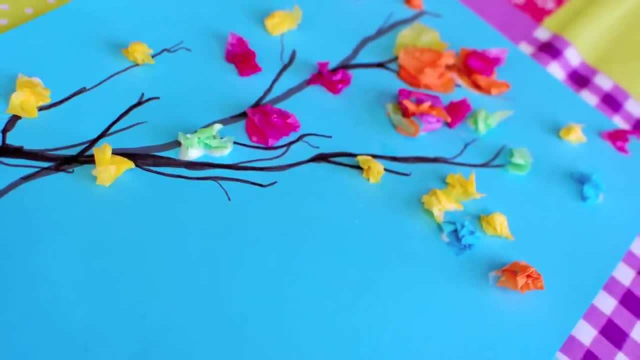 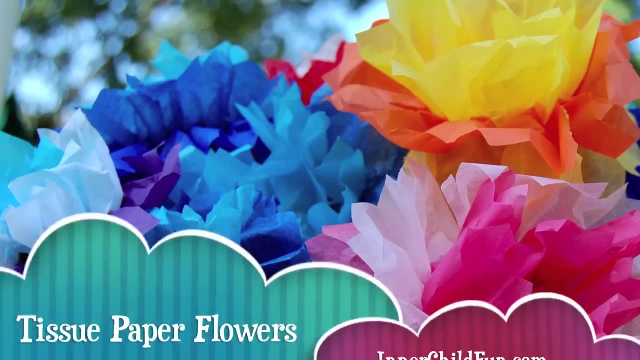 get really good results with a nice spring project that you can display in your house. The next project are these really beautiful spring flowers. They're made of cotton. They're made out of tissue paper. What I like about them is it keeps the kids busy and it makes. 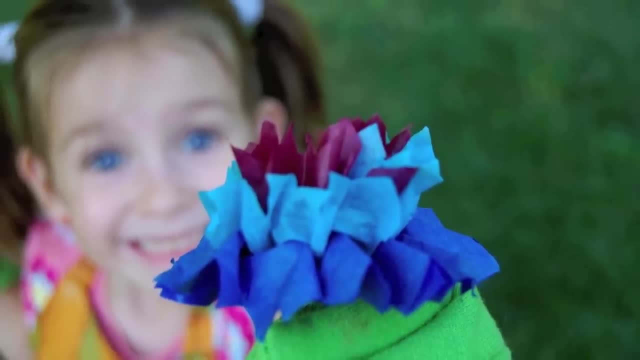 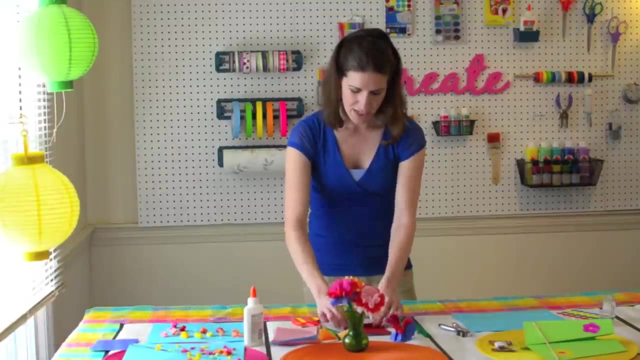 a really nice gift. So my daughter and I made a whole bunch of them one time and delivered them to the local assisted living facility. Really great way to introduce kids to gift giving and volunteerism. First thing I did was take maybe three or four sheets of tissue. 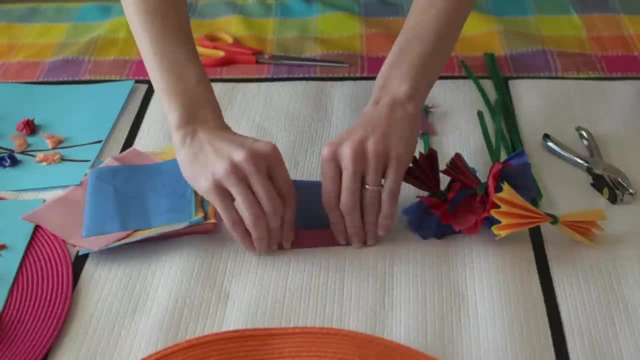 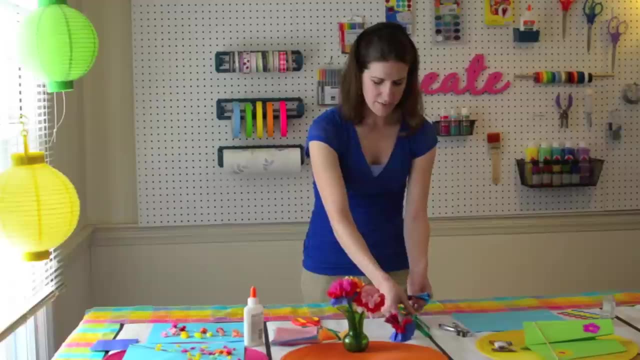 paper about the size of a large index card And we're going to fold it like an accordion. When you get to the end, just take a pipe grid And we're going to fold it like an accordion cleaner and wrap it around the middle, just like this. 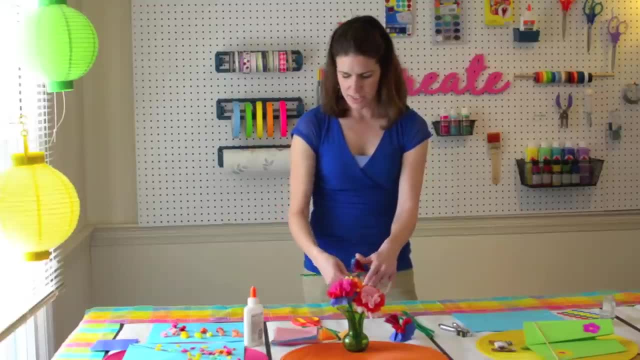 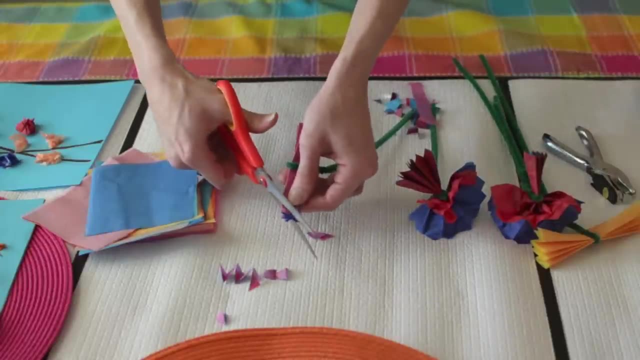 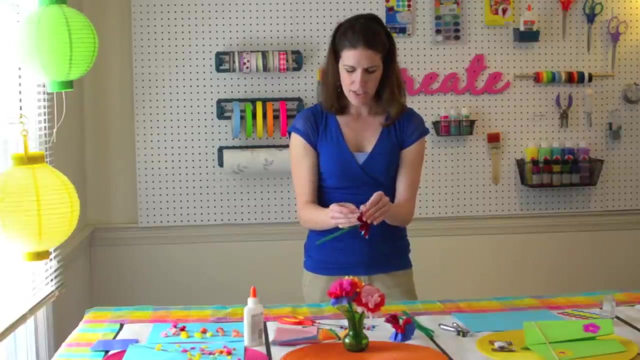 So quick and easy- and I love how spring-like these are. And then I'm going to take my scissors and trim off the ends just to make it really pretty. a nice clean finish, simple. And the last step is just to open up the flower and go ahead and very carefully separate the. 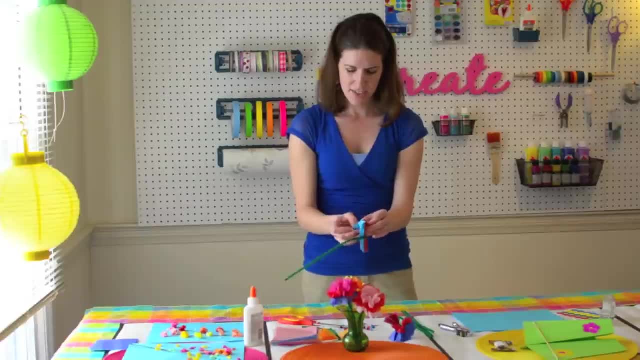 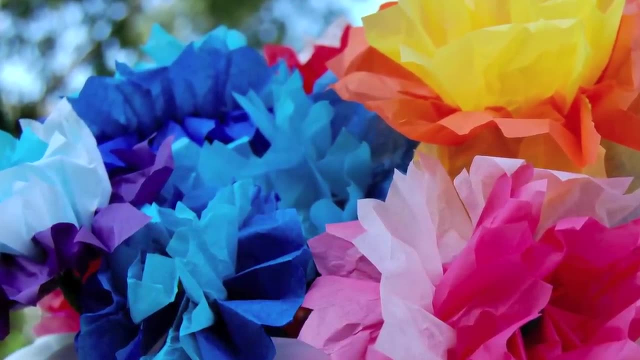 layers. This is good, fine motor practice too, for little ones. So here are the finished ones when they're all done. aren't they pretty? I think these are so much fun. The last project is a fun one to do outside, especially if you're at a playground.